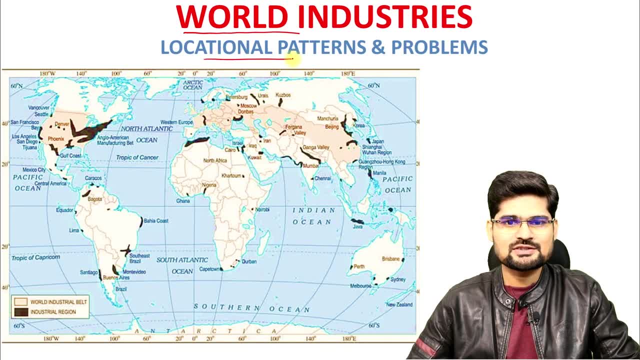 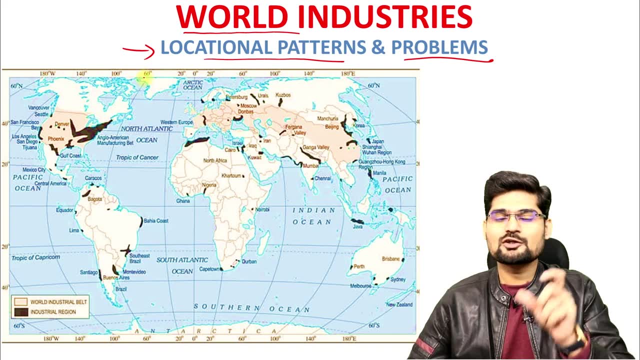 So now let's look into the world industries, its locational patterns and problems. Now, whenever we say locational patterns is essentially human geography, as we know. So in economic geography it has a very special position. Now, if you look into this map of the world industries, you will find where geography 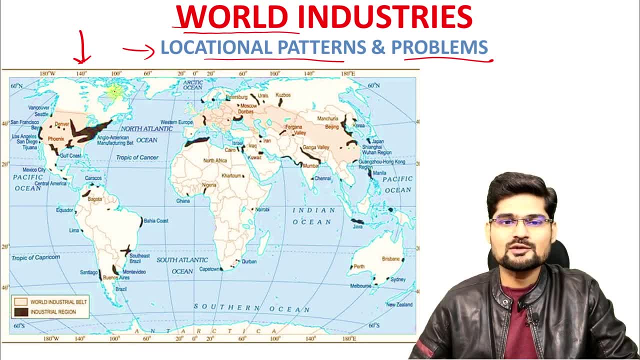 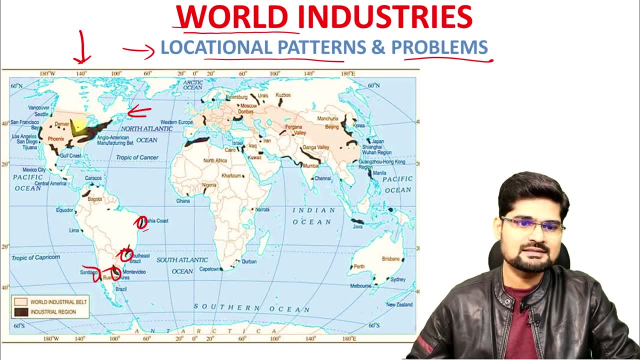 lies in economics. So look at the geographical pattern of these industrial hubs across the world. If you observe in Americas, north and south, you can find out. all the coastal areas are essentially the industrial belts. and then come to Europe. So again, some dots and some. 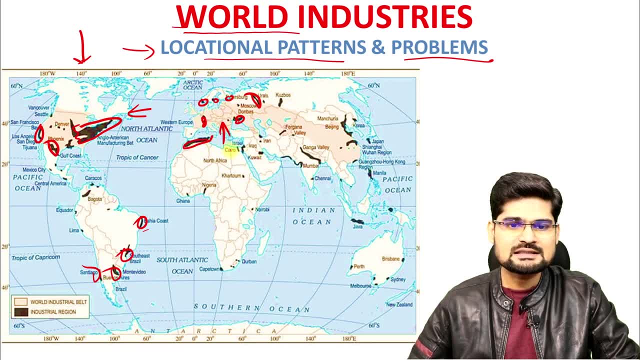 elongations. if you find north of all Mediterranean and some places also in south of Mediterranean, across the Asia Minor, if you find The South Asia, Southeast Asia, which is the modern hub of all the industries. if you find right in Australia, you will find on the coastal belt in India, across the northern 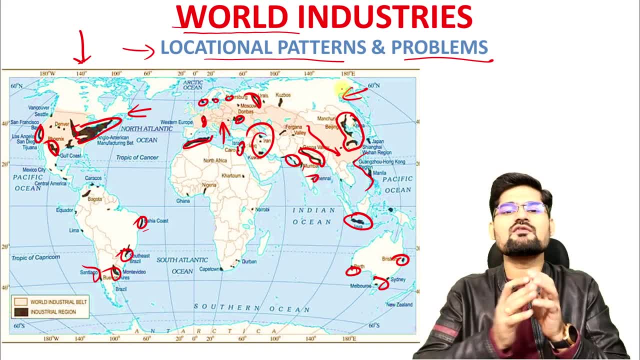 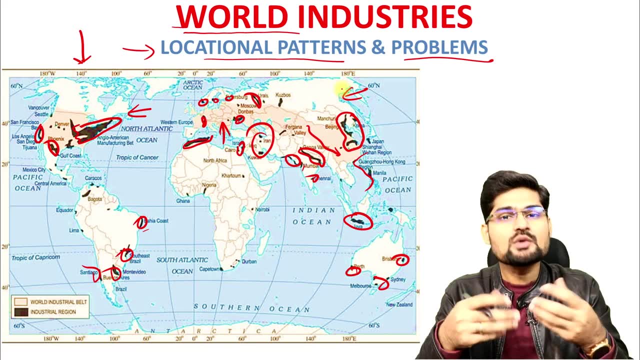 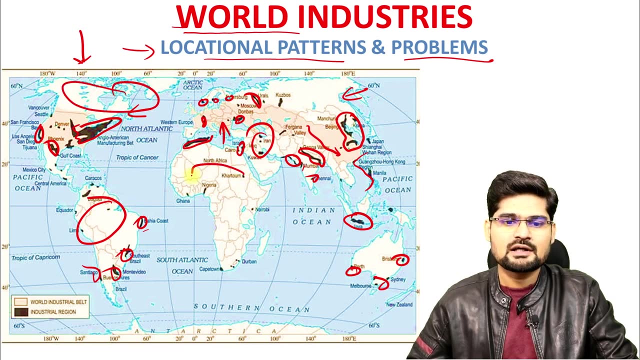 and the southern belts right. So this is where the location of all the industries are across the world. Now, if you find out, there are many more areas in the world which do have potential, but they are not industrialized. Several areas across the world, across Americas, if you observe, across Africa, if you observe. 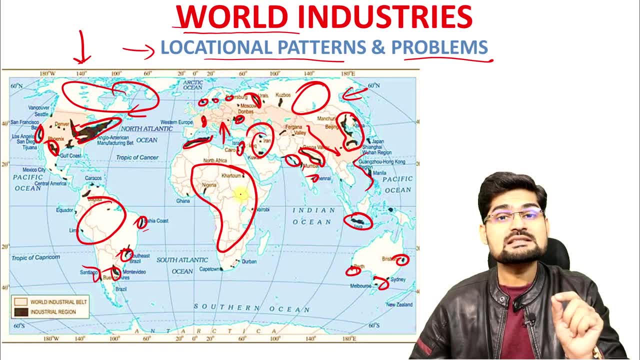 Russia, if you observe, and several other portions of the world. Now, these are the areas where industries are not there, where sustainable resources are not available, laborers are not available, other factors of productions are not available and also there are several socio economic factors because of which these areas do not have industries. So there is 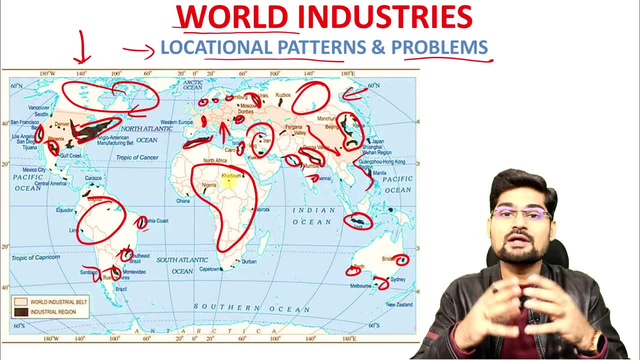 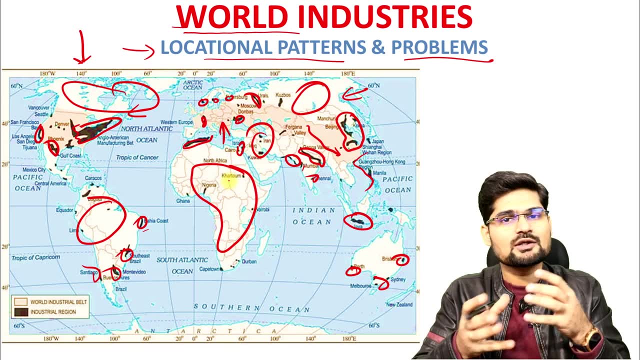 a distinction between the industrial located areas where we have also learned in models and theories: the industrial location theory by Weber, where he discusses all the factors related to it. you can go there and watch it again and understand why this pattern has emerged out. But here in 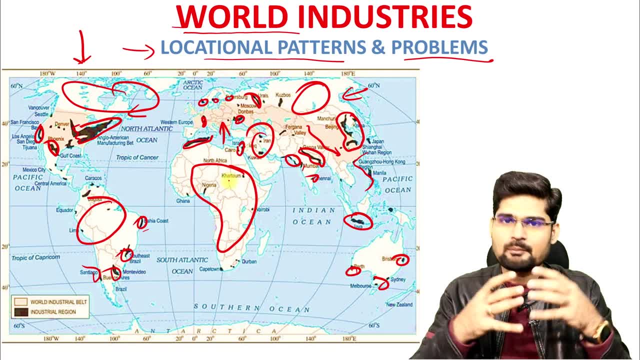 today's session we are going to look into the problems of these industries as well, and also look into the some of the areas where the factors of production and modes of production have resulted in the industrial hub creation across the world. So now look into the first part, that is, classification. 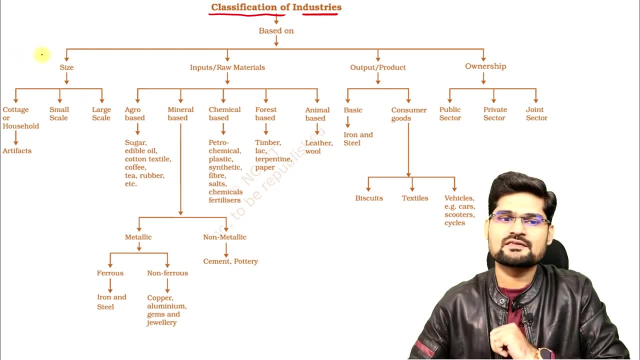 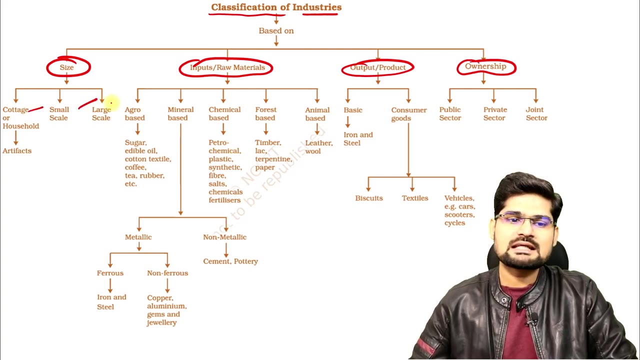 of industries. So there are bases of industrial classification, for example size, input of material, output of material and also the ownership. So four basic criteria to actually classify various kinds of industries across the world. So cottage, small scale, large scale. on. 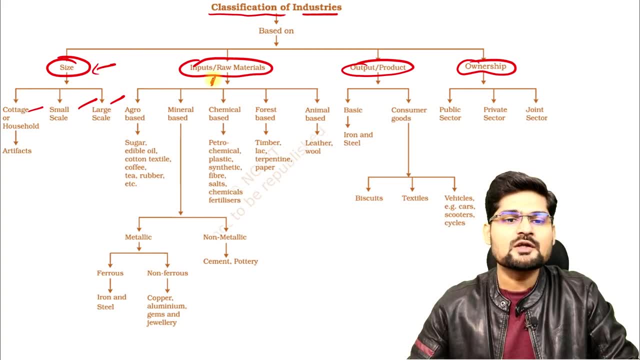 the basis of size. the scale factor comes there Now, in terms of inputs, industrial inputs, as factors of production. So agro-based, mineral-based, chemical-based, forest-based. you can find out several examples across the world and India, metallic and non-metallic, as well. on mineral, 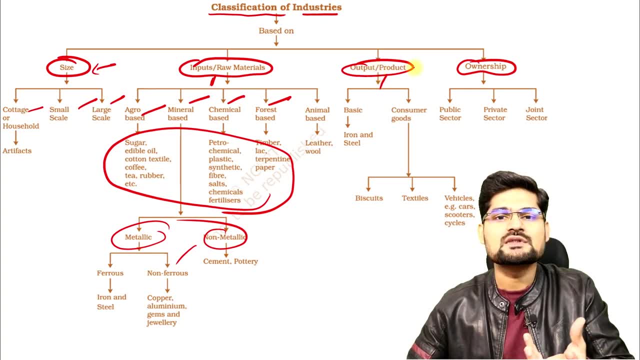 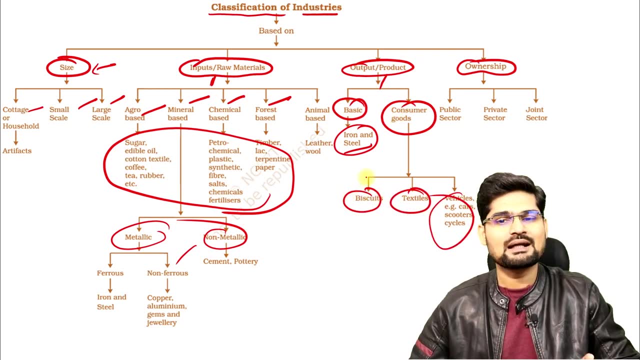 Then output what they actually process and produce, So basic that- iron and steel and consumer goods, for example biscuits, textiles, vehicles and several others. And apart from that, the ownership: who owns it? Is it a public sector or a private? 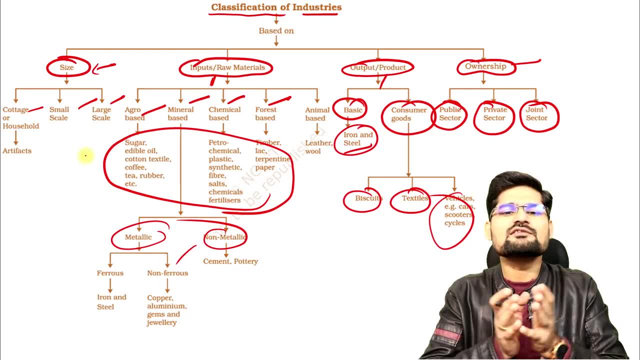 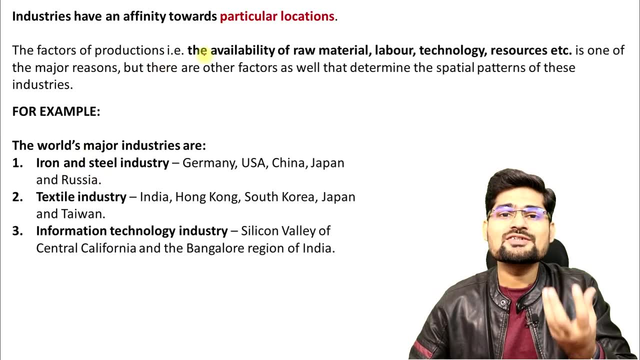 sector or a joint ownership. So these are the various ways of looking into the classification of industries across the world and India. Now, what is important here is the locational factor, the geographical factor, So industries have an affinity towards a particular location and that's where we talk about the location factor. So the location factor is the location. 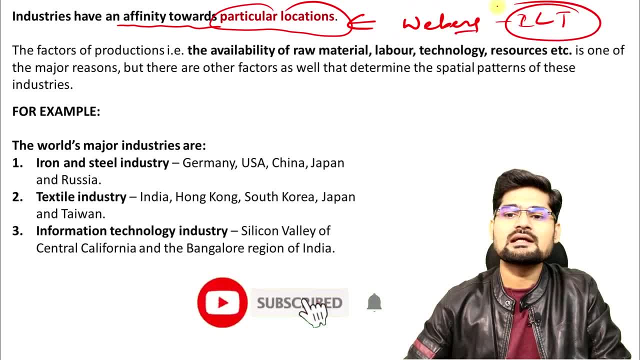 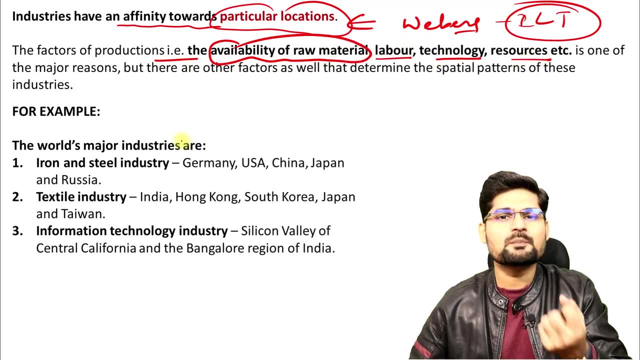 about the Weber's industrial location theory. So, factors of production, for example, availability of raw material, labor supply, technology resources, These are the four important pivots which lead to the creation of an industrial hub in a particular given space and time. 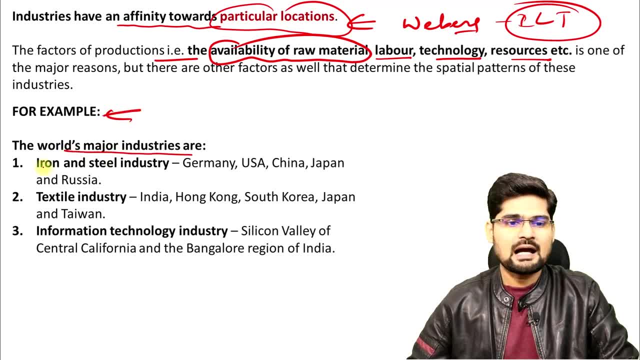 Now, for example, if you observe world's major industries- iron and steel industry- located in Germany, USA, China, Japan, Russia and also in India, if you find out, Then textile industry- India, Hong Kong, South Korea, Japan and Taiwan. 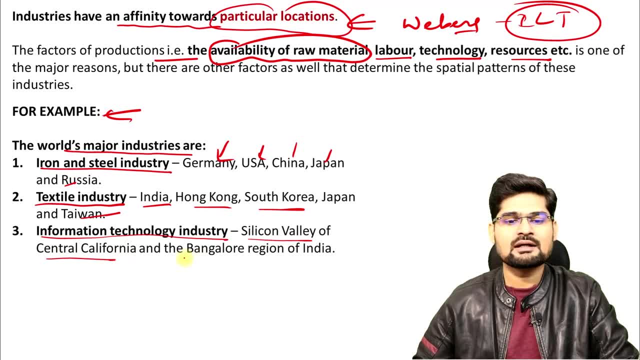 Then technology industry- Silicon Valley- very famous- the central California and Bangalore region of India, and also Delhi, NCR IT hub, Hyderabad, several other places in India. you'll find out. Then, why are these concentrations in these particular beds? That is the question. 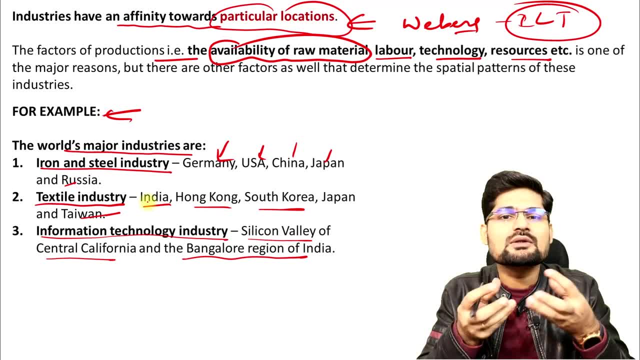 right Why there is a geographical pattern in this, Why there is a locational pattern in the establishment of these industrial hubs across the world. So that's where Weber industrial location theory and factors for industry establishment comes into the picture. Now let's analyze. 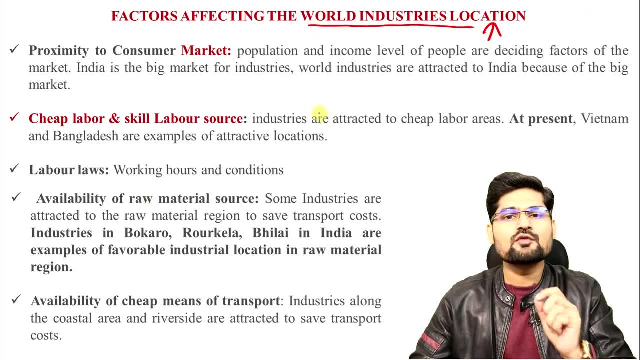 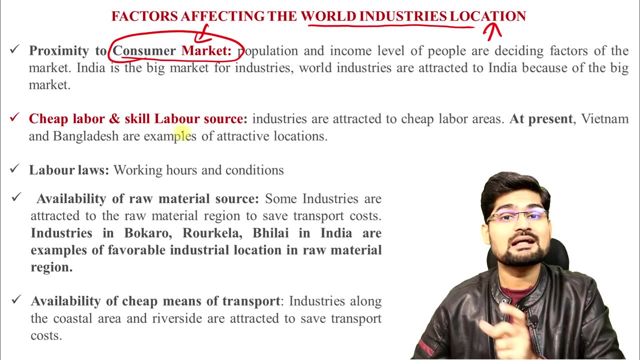 the factors affecting the world industrial location if you want to look into their problems, because the problems are associated with these factors. So proximity to the consumer market is the first factor if you observe that who is going to consume the products coming out of the industry That deals a lot. Market has a very important value in terms of when. 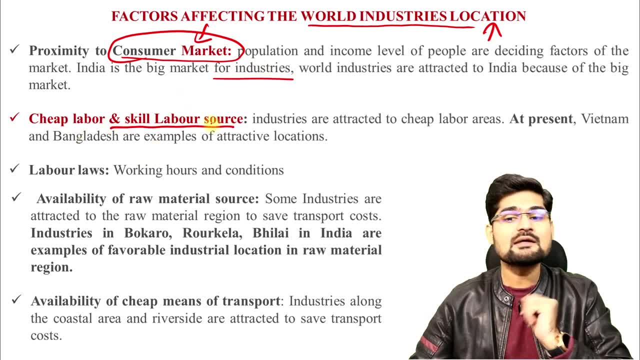 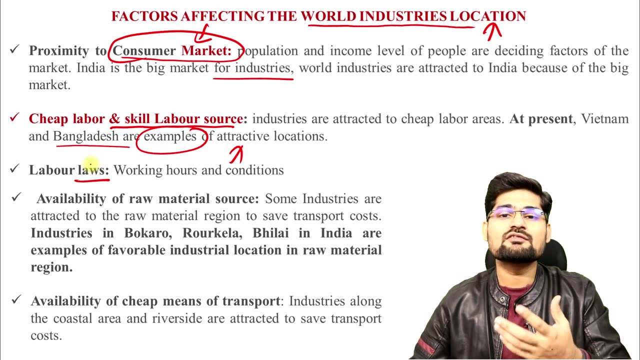 we set up the industries across the world. Then cheap labor and skilled labor sources very important. So countries like Vietnam and Bangladesh are doing well as attractive locations. Then labor laws. Now it all depends upon what kind of facility is government giving to the laborers and also what kind of laws are governing the work condition of the laborers. 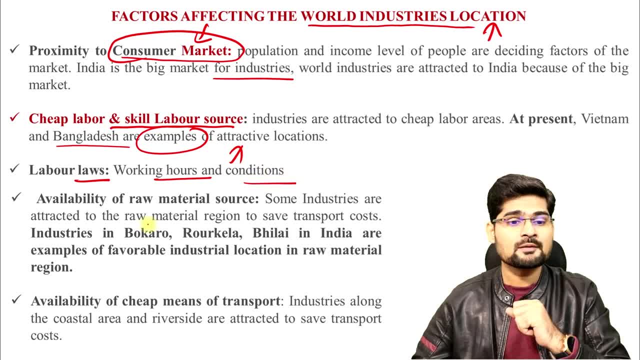 right. So working hours, their conditions, these become really important. Availability of raw material sources: Obviously it's very important because you have to produce, you have to have input. So in input, raw materials really become important in terms of industry. 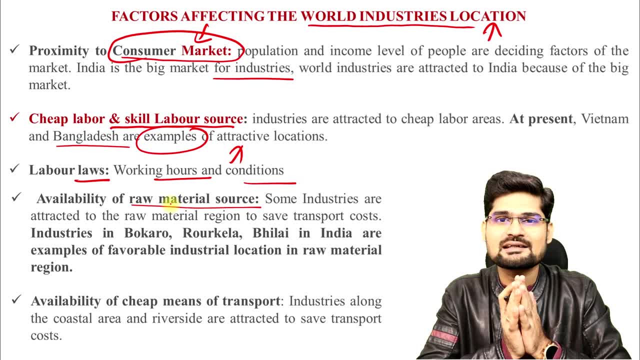 establishment. For example, if you look into the iron and steel cities in India, they are all mostly concentrated. They are located in the mineral belt of India right. So that is where the determinant factor arises: Raw material, the iron ore right And various other ores, which is important. 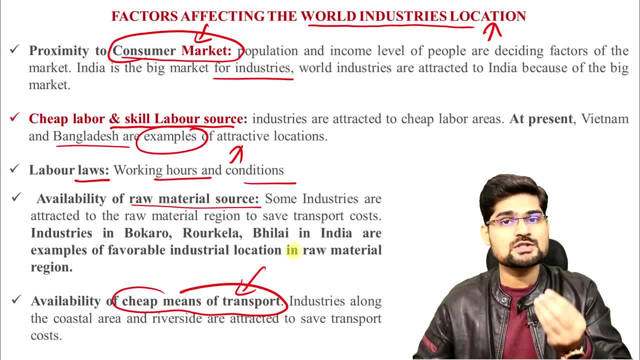 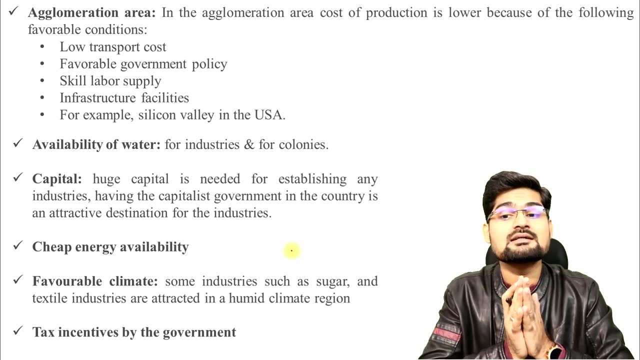 Then availability of cheap means of transport, because transportation is which will carry the input linkages to the industry and also the produce to the market. So transportation becomes the lifeline of these industrial setups. as we have already discussed in Weber industrial location theory as well, Now agglomeration areas In the modern economies, especially 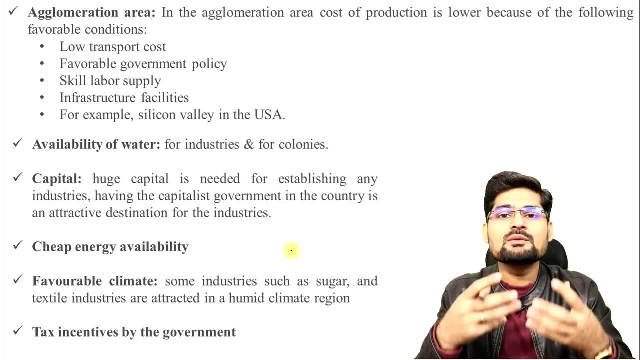 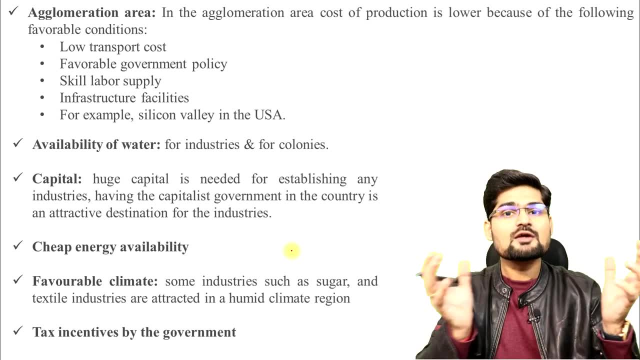 the post-World War II economies. if you observe, the agglomeration areas play a pivotal role. Not a single area in isolation can develop as an industrial hub. So agglomeration of factors become really important right. So: low transportation costs, favorable government. 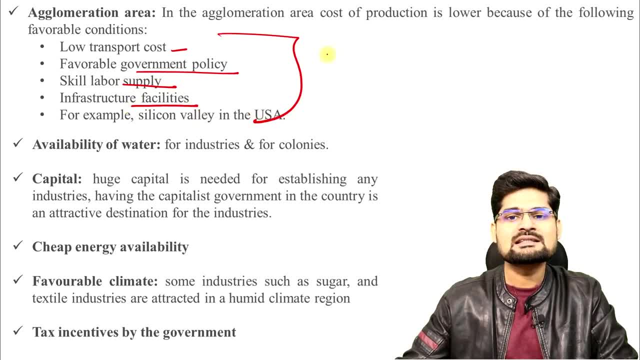 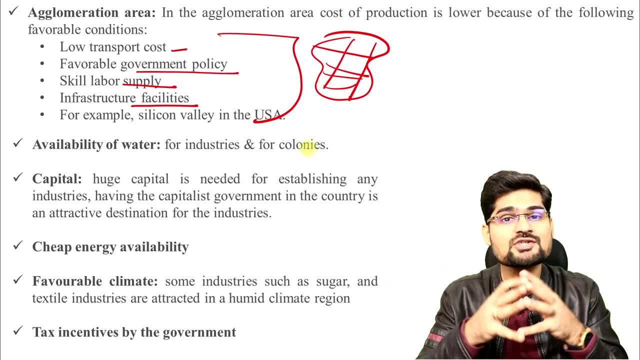 policies, skilled labor, infrastructure facilities, all these things in a particular region makes it an industrial hub. So there is an aggregation of the factors, the combination or agglomeration of the factors in one particular area That is important Now: the natural resources which are important and some of the important natural resources. 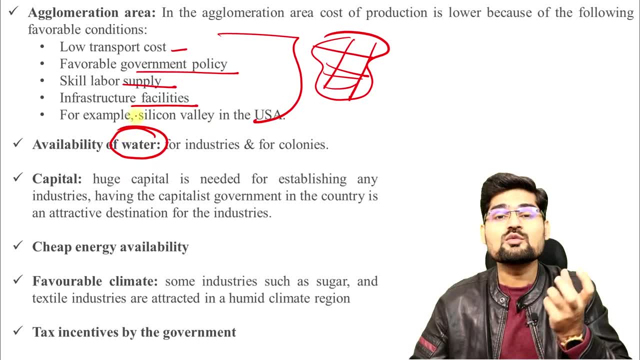 for various industries is the availability of water. Without water we cannot thrive. in terms of industrial setup, In most of the cities and all areas in the world, if you have observed across industry, availability of water becomes really important. So, even if water is coming from the underground sources or from the canals or from the river water, 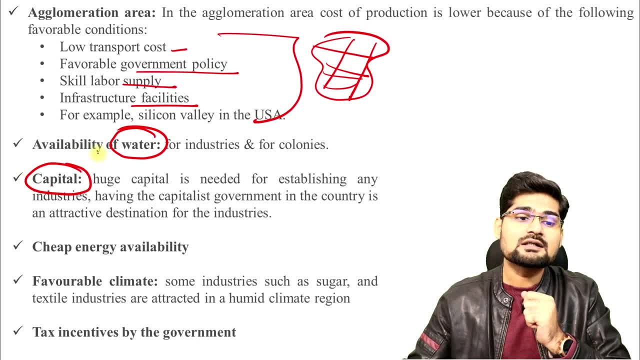 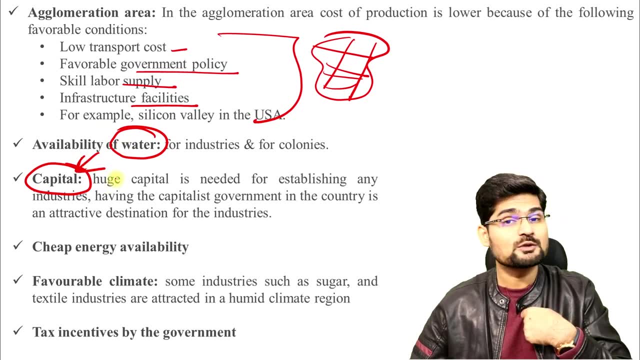 source becomes really important. Now capital. Here comes the important part. Capital is an important thing. Finance, the capital, the money, which is important. If you remember, we have talked about this in growth pole theory as well. right, The multiplier effect is created. 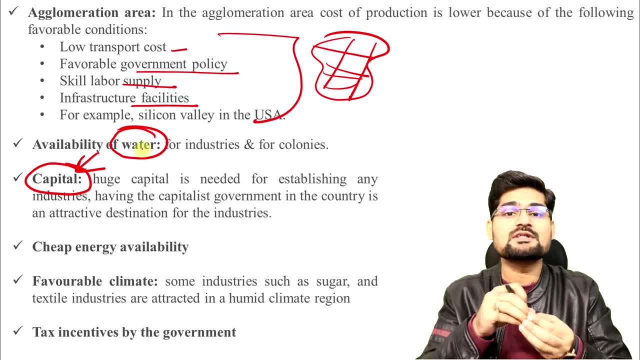 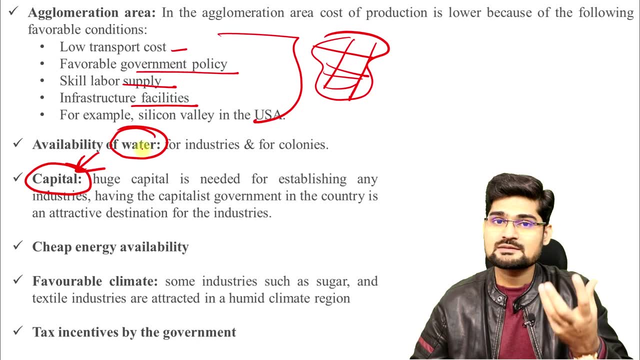 by the corporates, the big industrial hubs. When they establish themselves in one area, they create a multiplier effect across their society right. So that's where capital intensive work is very important. So capitalists are the backbone of industrialization across the world, and they work in tandem with the government, So it's very important to be an agglomeration. 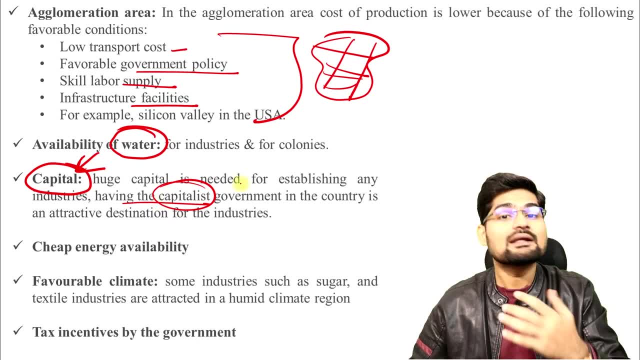 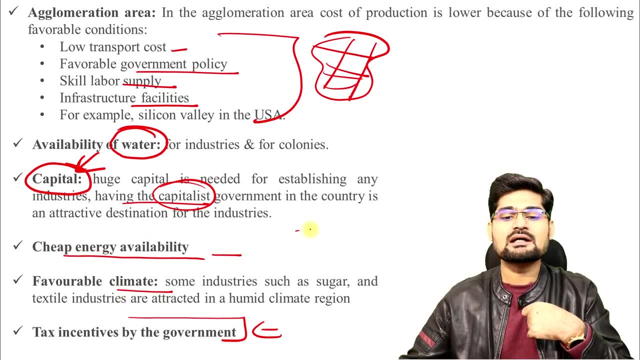 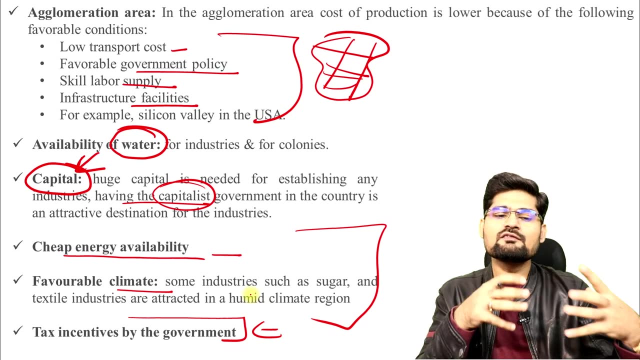 If you want to industrialize, that is still the policy Now. cheap energy availability, then favorable climate, tax incentives by the government are several other factors that also determine these locations of various industries across the world. So now, when we know these several factors associated with industrial location related to Weber's industrial 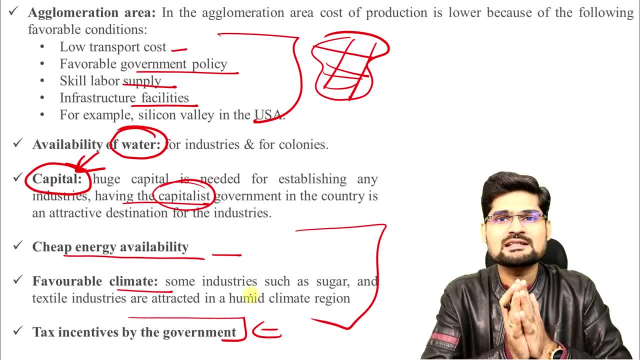 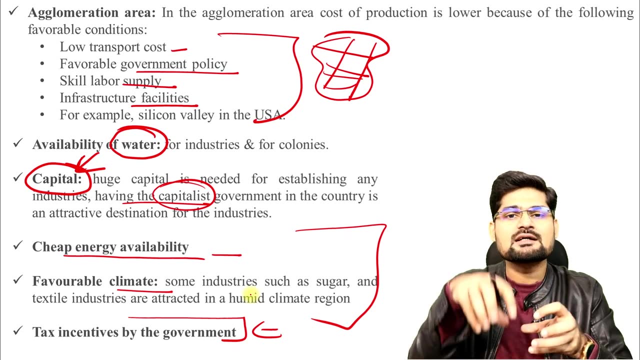 location theory or growth pole theory and several other industrial theories. what we understand is: these factors are not spreadable. They are spread uniformly throughout the world. right, The growth does not happen in uniform ways. So we have the polarities, we have the locational areas, we have the important dots. 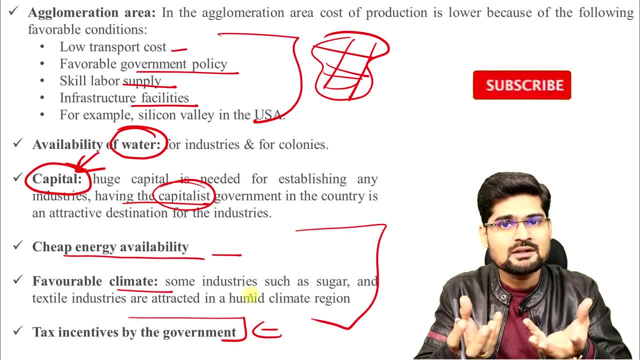 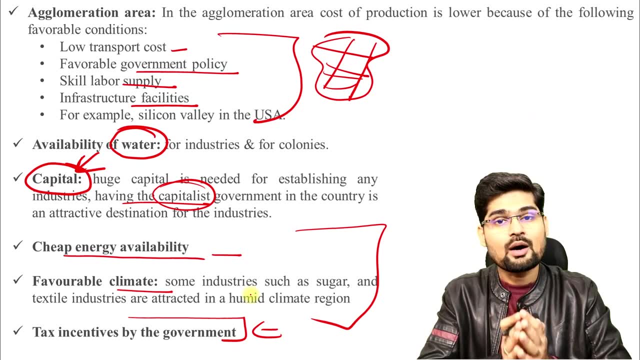 on the world map where you find these facilities available, And that's why the industrial hubs in a better condition in those areas and other areas are devoid of industrial location. Now with this is linked the industrial problems. So first of all let's look into the analysis. 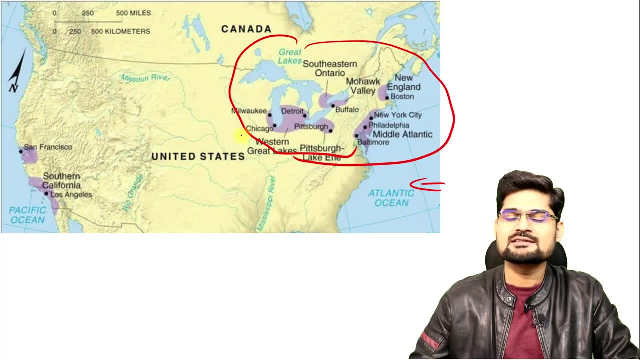 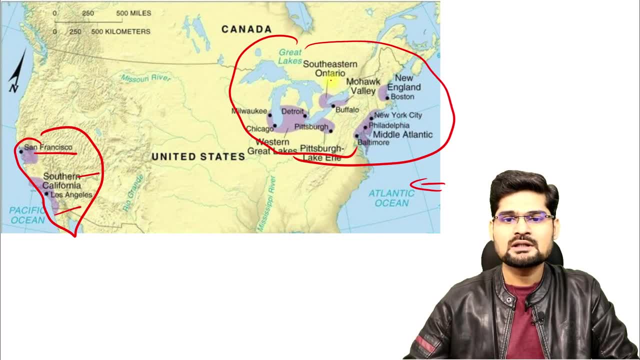 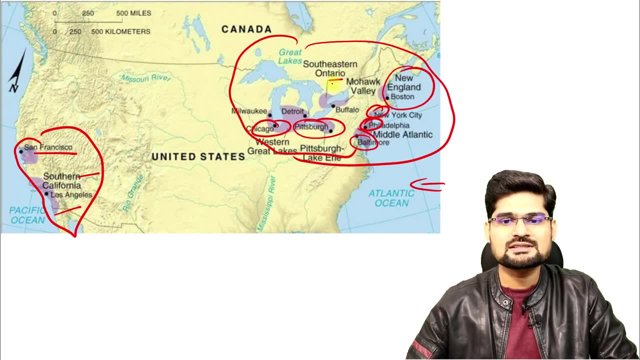 San Francisco, Southern California, LA, and also here the Ontario, the Great Lakes region here, Pittsburgh, New York City, Philadelphia, Baltimore and so many other areas in Boston and other places. right, These are the industrial hubs here. Now look into the European side. 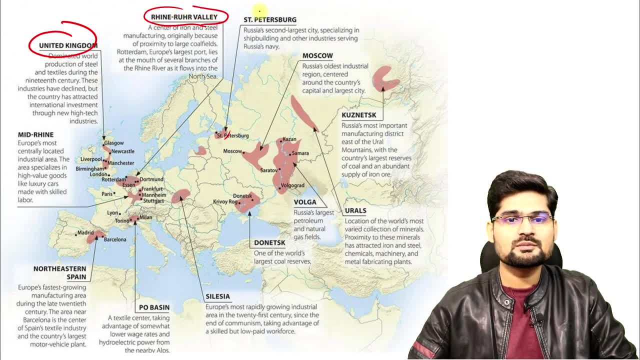 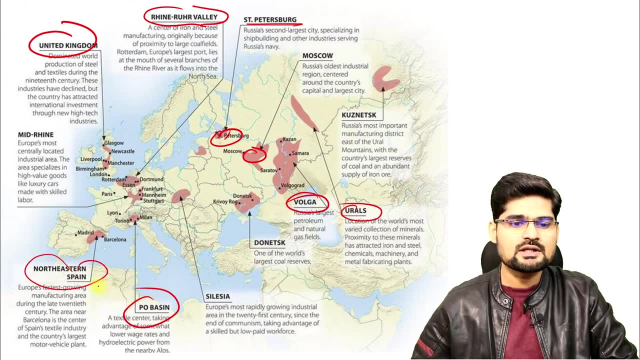 So United Kingdom Rhine-Ruhr valley. if you know here in Germany St Petersburg, then you have in Moscow right Ural Mountains, Volga region And several other industrial, several other region, Po region and Spain. If you observe the world map there is in. 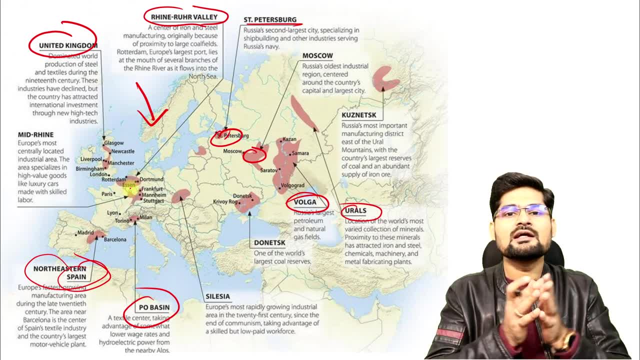 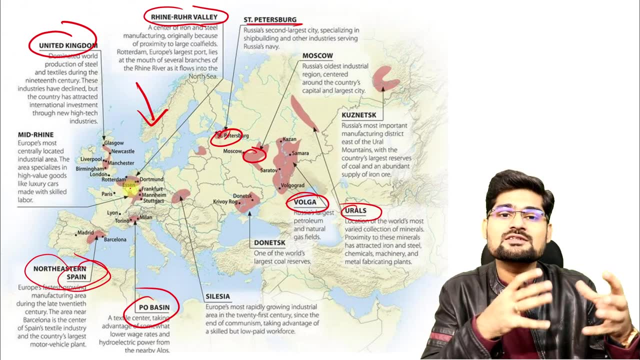 Europe and also in some portions in Russia. If you find, the Eurasia region has a lot of areas where industrialization is there because of natural resources and also because of the historical reasons. These were the hubs of city-states, mercantile states. If you observe the Western Europe, if you 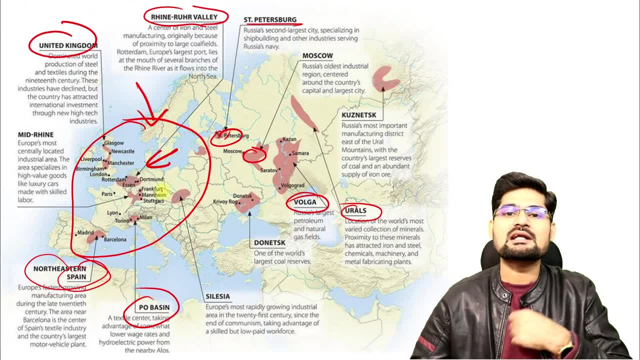 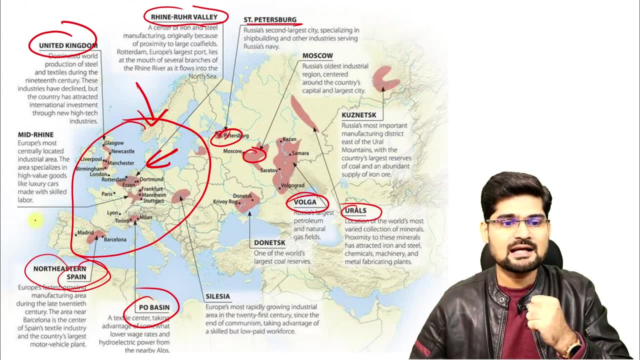 know the geographical thought here, the first kind of trading towns and mercantile city-states developed in the Middle Ages and also some of them right from the ancient, because they had open ocean- Here you had Mediterranean and they traded across the Gulf. So these areas had all these locational 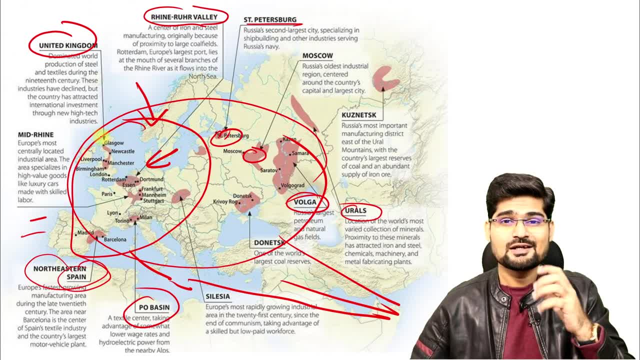 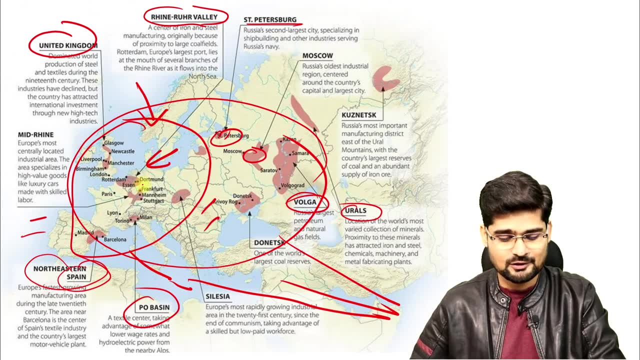 importance. I am talking about geographical importance here. So geography played a very important role all throughout the history- and still playing- in terms of the development of these industrial hubs across. Now look into the China side and South Korea side, where you have industrialization in. 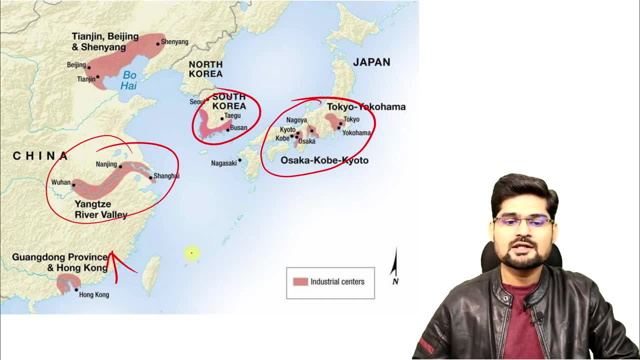 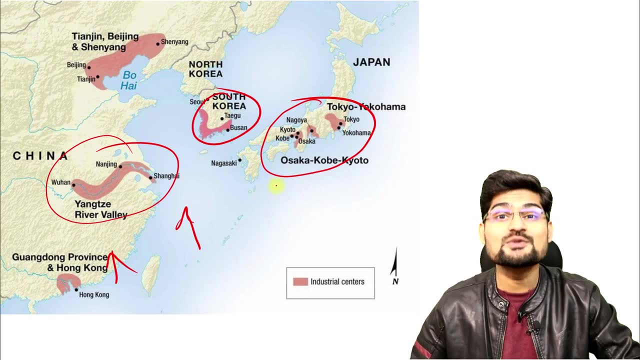 Japan, South Korea, China, etc. These are the important areas. You can take this map, you can pause the video here and look into these particular areas where the modern industrial setups are there, special economic zones are there and how China is leading the world chart in terms of the industrial production, because 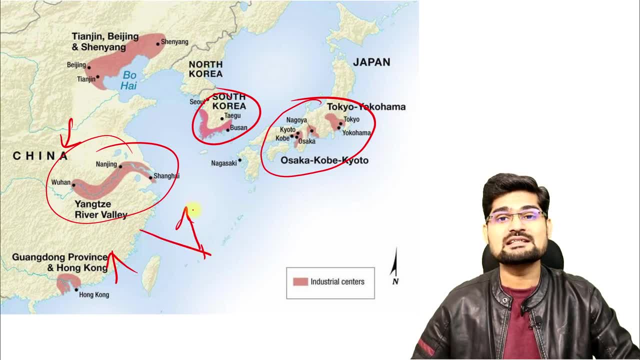 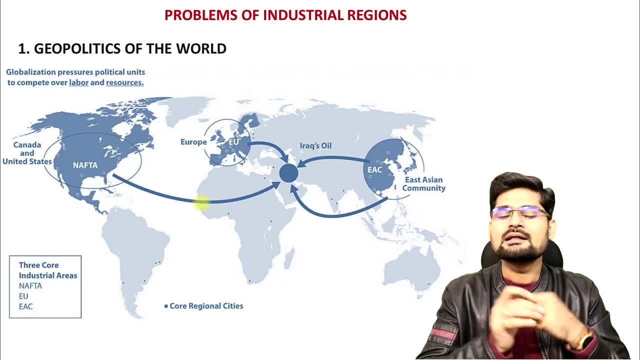 of the land, labor technology, access, transportation facilities and everything which is agglomeration in one particular area. That's why it's very important Now, because we know the world pattern, it's important to also look into the problems of industrialization or industrial regions across the world. 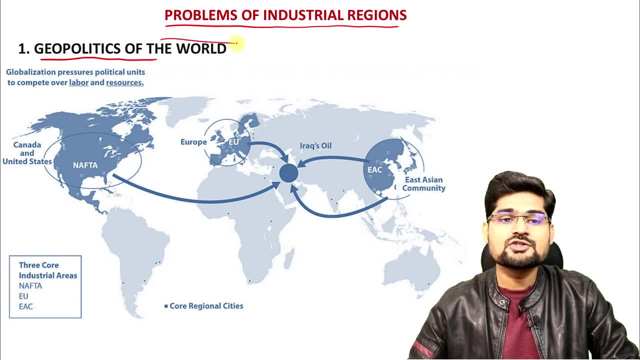 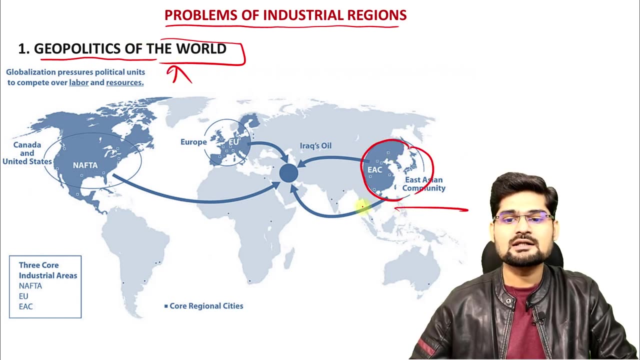 The first important thing is the geopolitical issues or challenges across the world. The world has been, and always since ancient times till today has been, aligned across the power structure and that is dealt with the economies. So if you look into the modern world now, remember this East Asian community in. 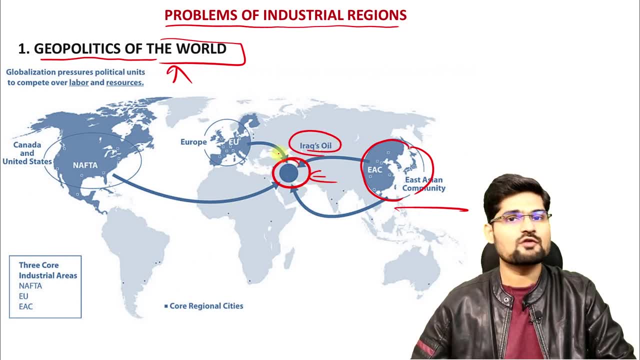 the Central Middle East, you have Iraq's oil and several other areas where you have OPEC countries. then you have European Union and then you have this Canada and USA. So these are the core regional cities which you observe as NAFTA, EU and EAC, which deals or has the control over world. 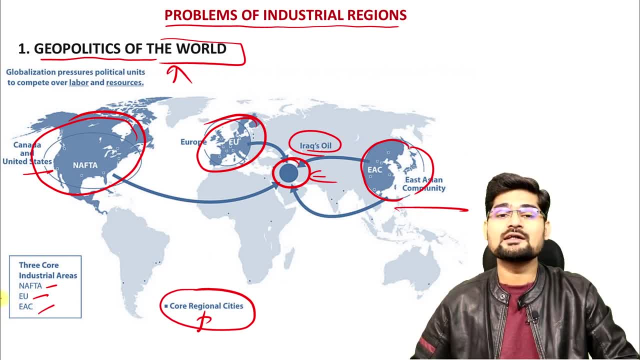 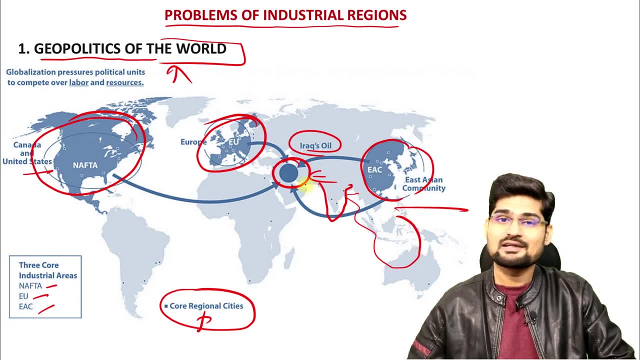 economy mostly, and that's why they dominate the world in terms of decision making. We also have SARC nations, which is not that effective. We have Association of Southeast Asian Nations and we have several other units of trading across the world. But what is happening? because of geopolitical 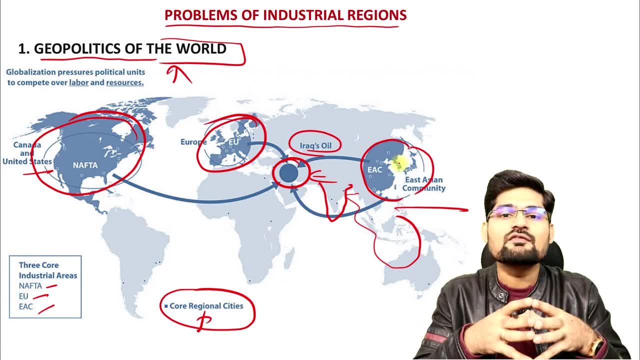 tensions, issues, political instability, the problem of industrialization still persists. Some dominates, some are being dominated. So entire class structures, organized structures, industrial structure management and infrastructure is still prevalent across the economies in the world. So geopolitics is one factor. 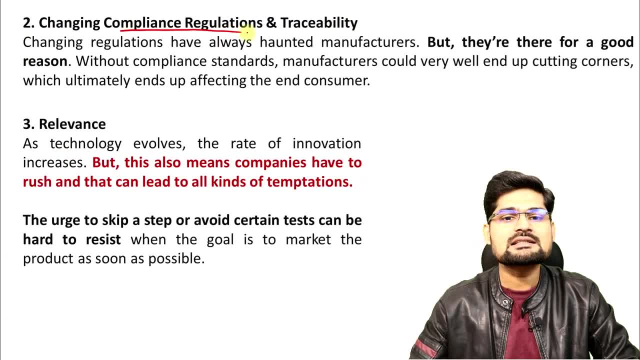 that leads to several problems across the world. Then, other factors- changing compliance regulations and traceability. This is very common to the manufacturers across the world, industrialists across the world, because, remember, there's several regulations which keep changing and the standards are also changing. 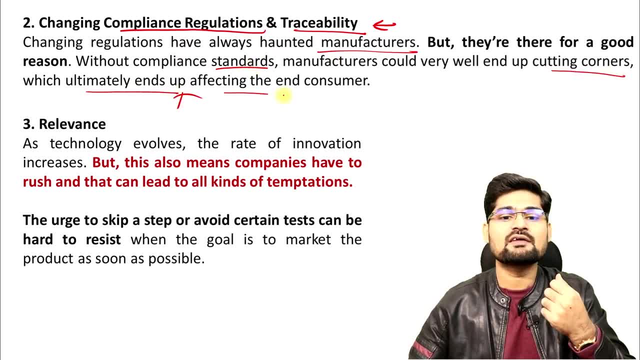 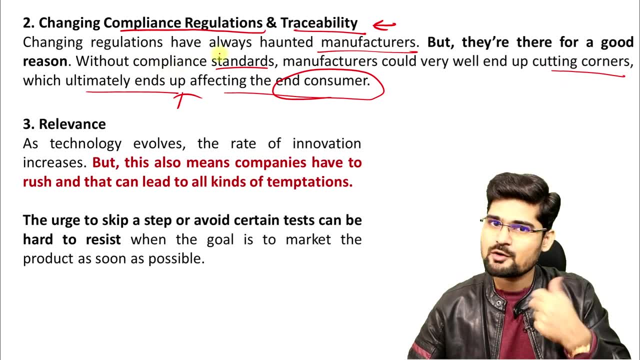 across the world. So manufacturers could well end up cutting the corners, which ultimately ends up affecting the end consumer. change in production standards and regulations keep changing in economies. there is a problem again to cope up with the demand and also the quality of product. then comes the relevance. 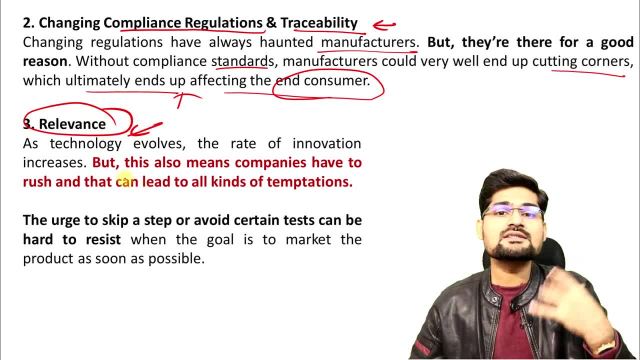 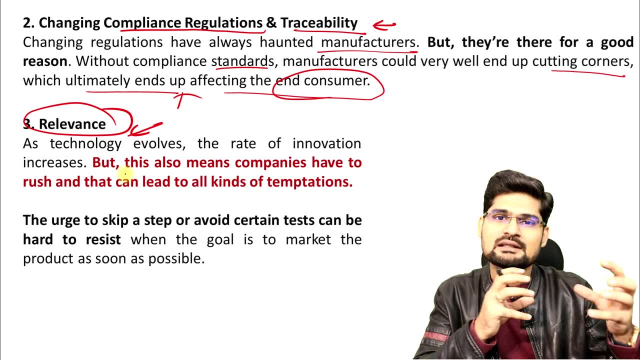 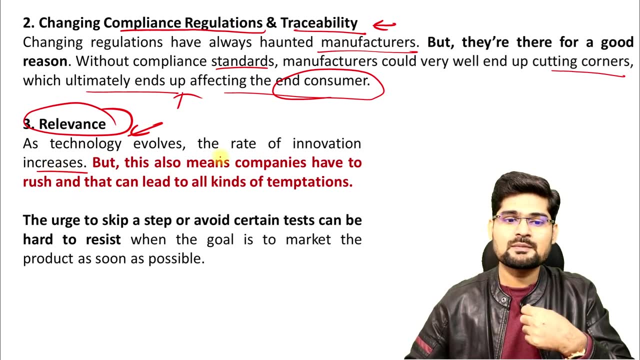 now remember, with technological changes, the relevance of industrial goods keep changing. if you look into the mobile phone technology itself in last 20 years, you will find the relevance of the technology has changed the market so much, right. so what happens? the rate of innovation increases with time, and what happens? the means companies have to rush, and that can. 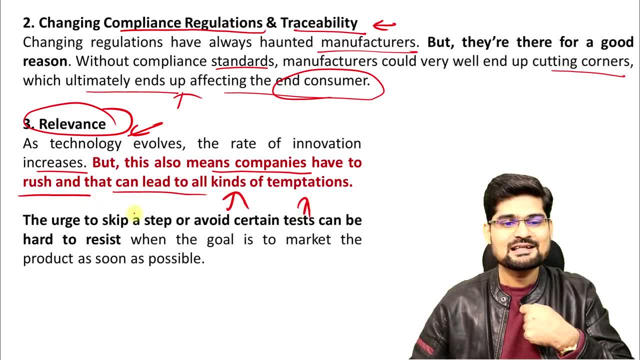 lead to all kinds of temptations. so what happens here? the urge to skip a step or avoid certain tests can have the problems across the system of industries, across the market. so this is a problem that everybody wants to make a profit in industrial setup. and what happens? because of the 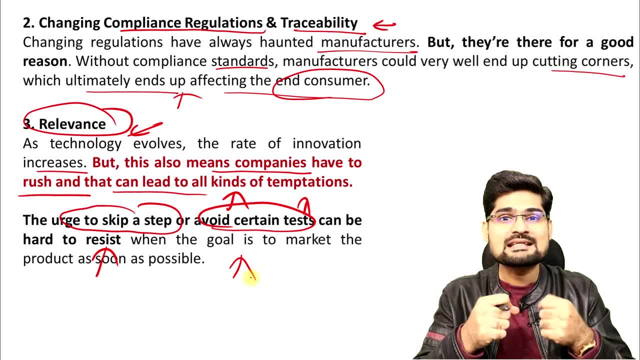 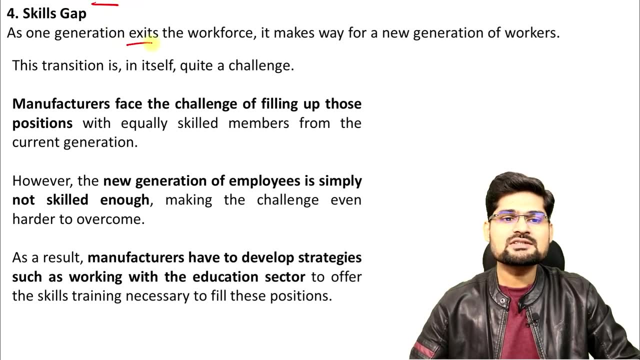 continuous change in technology. there is a race and across the race, there are so many things that are happening and you, so what do you find? next one is your skill gap. that keeps happening. now, remember, one generation exits the workforce and makes way for the new generation of workers. but what happened? the 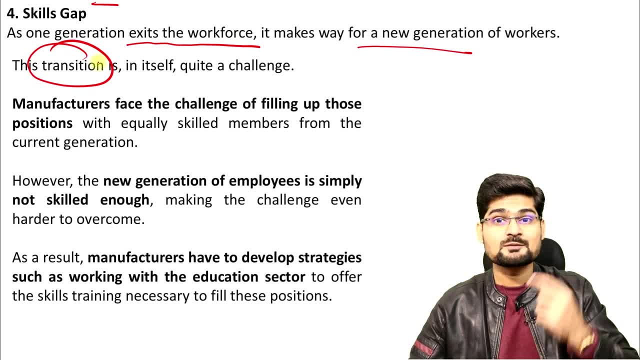 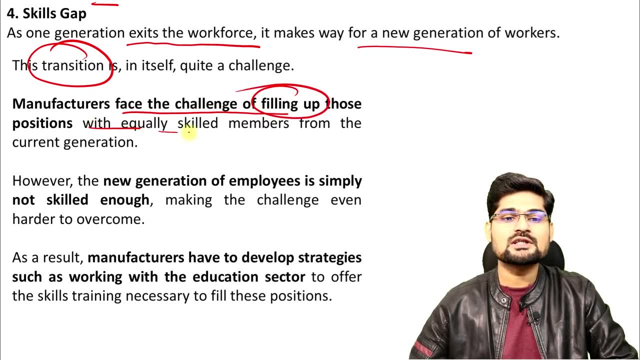 transition, the transition between the two generations in terms of technology is a problem or a challenge in itself. so manufacturers face this kind of challenge of filling up those positions with equally skilled members because, remember, experience is very important and production sites in industries right. so the newer force, newer employees are not skilled enough. they 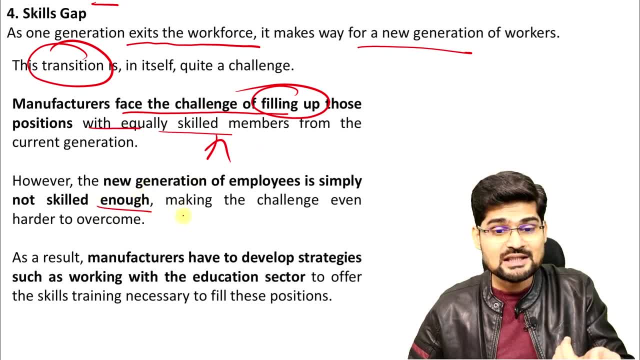 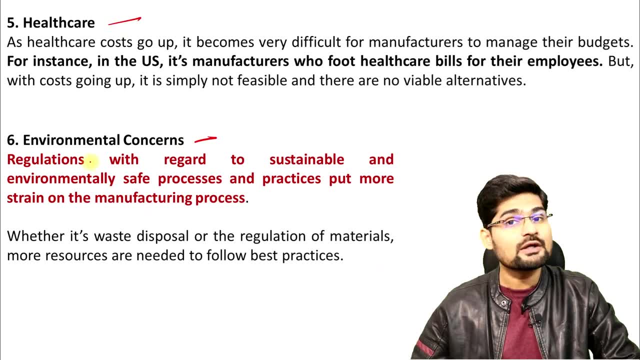 would take time. they would take training, so you have to invest on training. that's also a major challenge in today's world for the industrialists, and health care and environmental concerns are growing up across the world industries. if you remember in us its manufacturers, who put health. 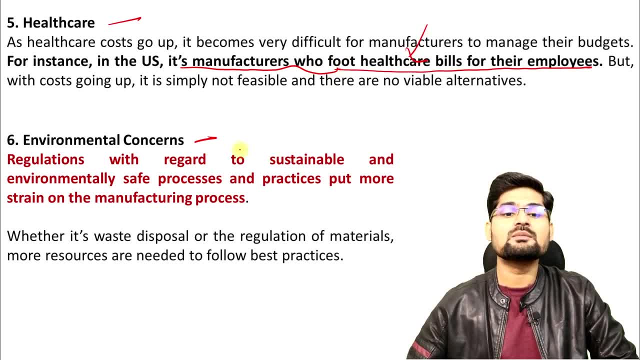 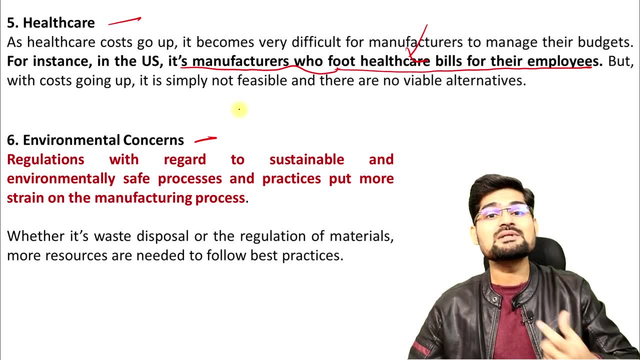 care bills for their employees. now remember, their health care bills are also taken by manufacturers in many countries. but remember, this is the industry that is the one that is most important. This is where cost goes up, so at the consumer end you will get the final product with increased 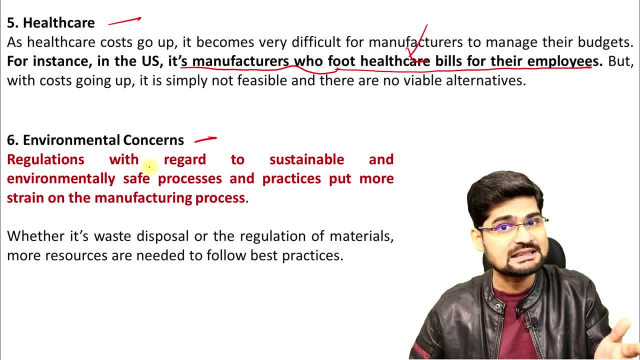 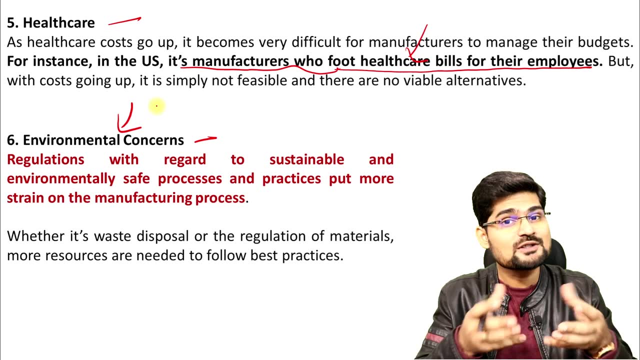 cost because of so many factors that are associated in the production chain. so health care costs have added up. now environmental concerns across the worldwide industry. whenever we say environment, remember it is directly looking into the industrial side. saying that is negative, isn't it? but without industry we could also not thrive. so what is happening? environmental concerns are growing. 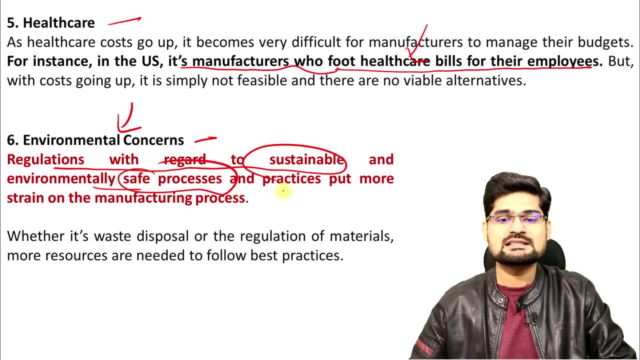 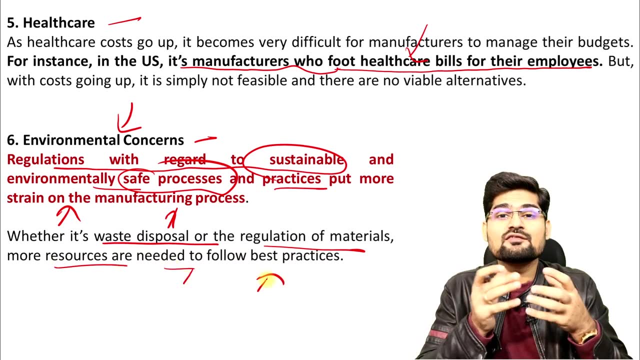 regulations with regard to sustainable and environmentally safe processes and practices put more pressure on manufacturing process because they have to take care of it. they cannot randomly keep producing goods like that, so waste disposal and regulation of materials and more resources are needed to follow the best practices, even if you know that eco-friendly technology in terms of 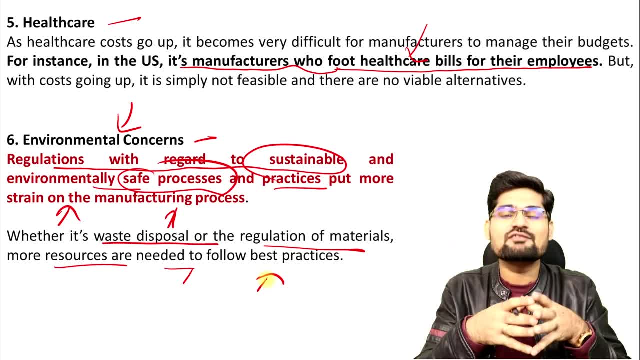 five-star ACs, three-star ACs and so many things that have come up across. modern technology in refrigerator ACs and modern technologies for our benefit, for the consumption of the consumer goods across the world. what has happened? there is a industrial chain that has set up. now they need to follow the guidelines related to sustainable. 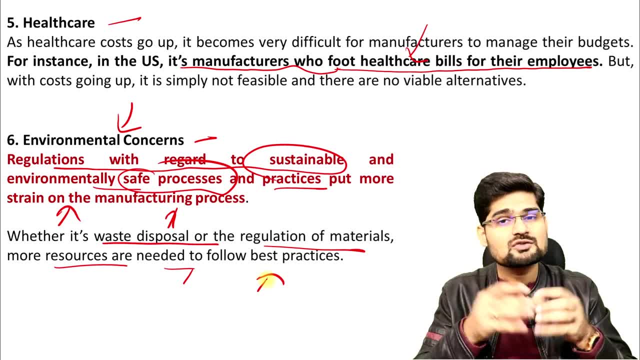 development goals. right in every country, there are regulations, so these are the challenges for modern industries across the world, and that's where we are looking into the economic geographies of these industries across the world and now, at the end, what we are looking at: the industries and 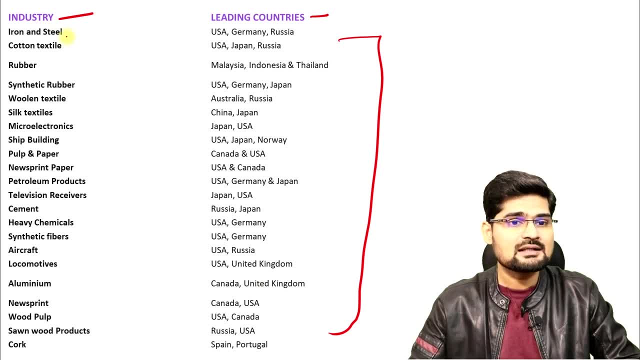 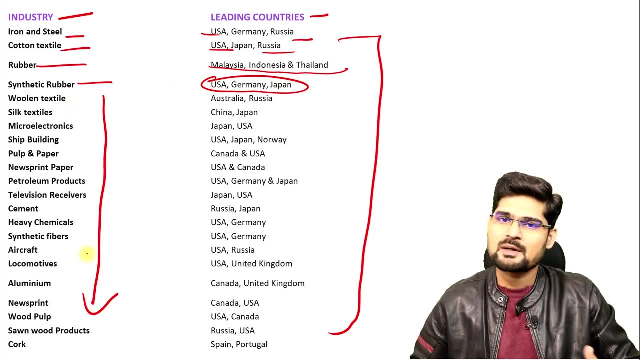 leading in terms of which kind of production? so iron and steel industry, USA, Germany, Russia, still leading. cotton textile, USA, Japan and Russia is leading. in rubber, Malaysia, Indonesia and Thailand is leading. then in synthetic rubber, USA, Germany and Japan is leading, and there is an exhaustive list that is here, which you can read by pausing the video here now. this is giving you a. 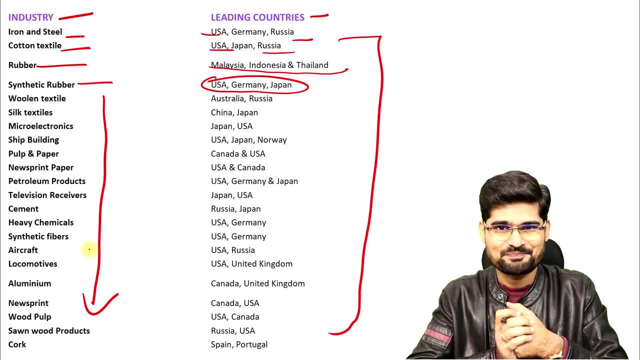 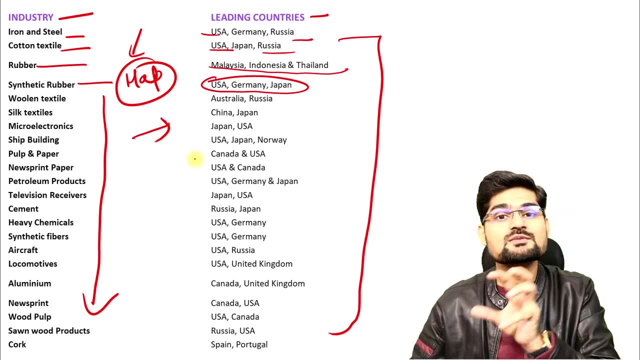 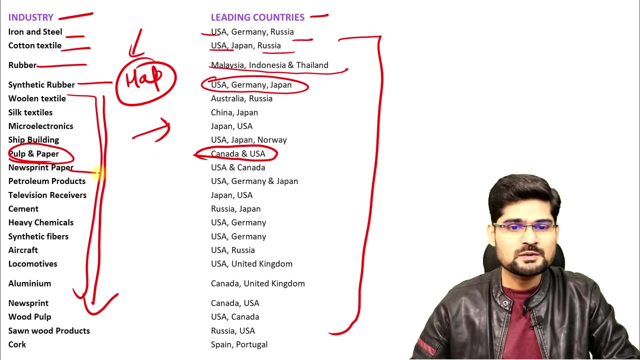 geographical pattern in terms of the production of goods- right. so what you can do is not just leave into a table, but you can make a map of this data, that where which is mostly produced, which kind of goods- right, for example, pulp and paper. Canada and USA is leading again. newsprint paper USA and Canada.